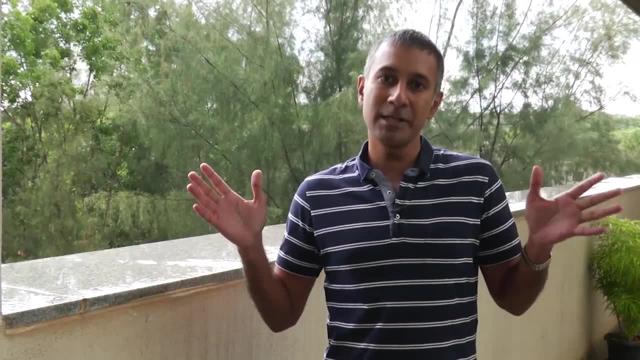 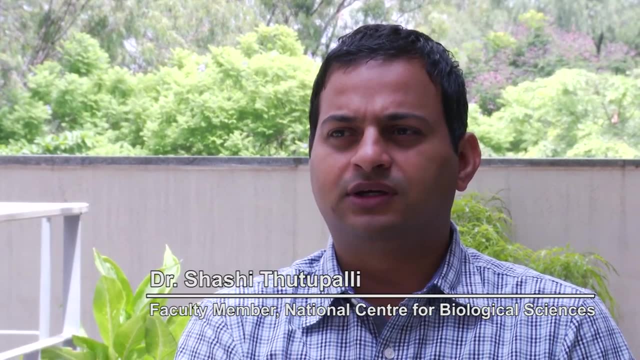 campus and expose them to all kinds of biology. It's a huge amount of information in a short span of 10 days or two weeks. This is the fourth year that we're running this NCVS Simons Monsoon School. It started in 2013.. It was started by my colleagues Mukul, 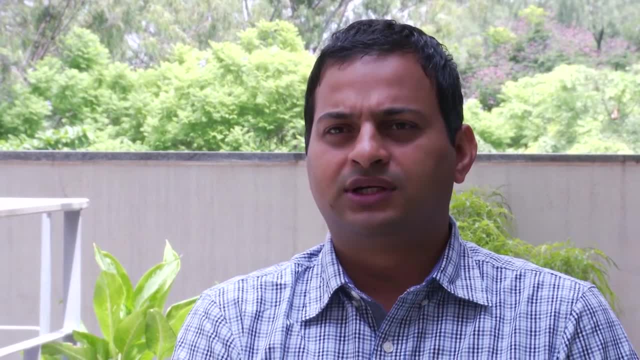 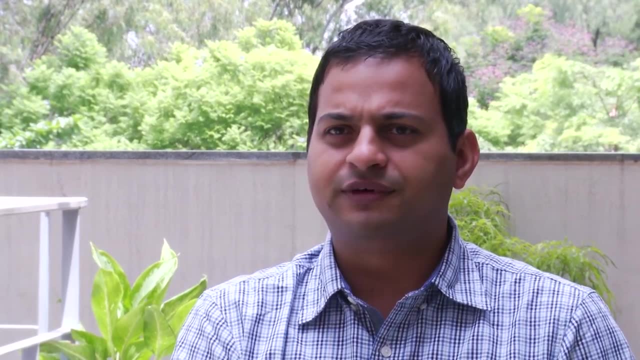 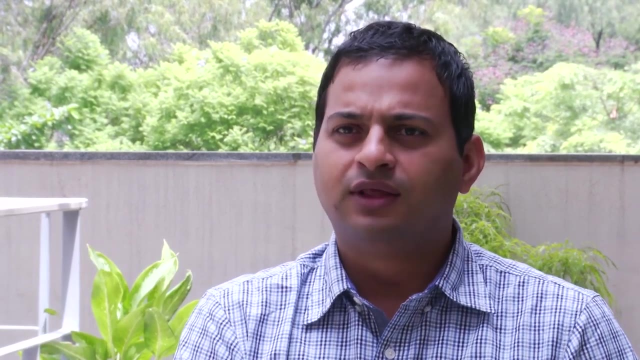 Kuntate, Sandeep Krishna, Madan Rao Shachi and Madhu Venkatesan at that time. And the number of applications: this year we got about 250 from again these various backgrounds And we go through a rather simple selection procedure after which we get about 40 students. 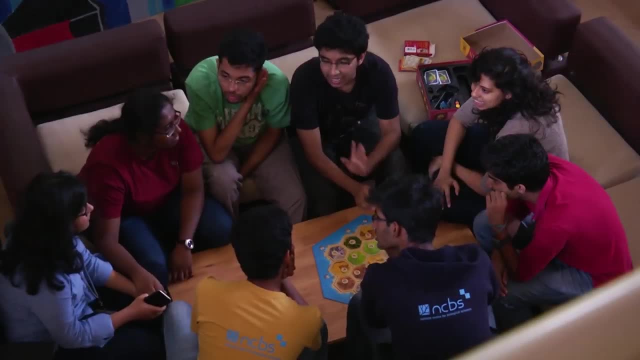 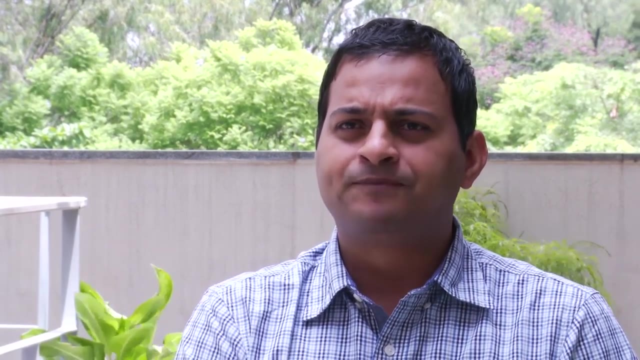 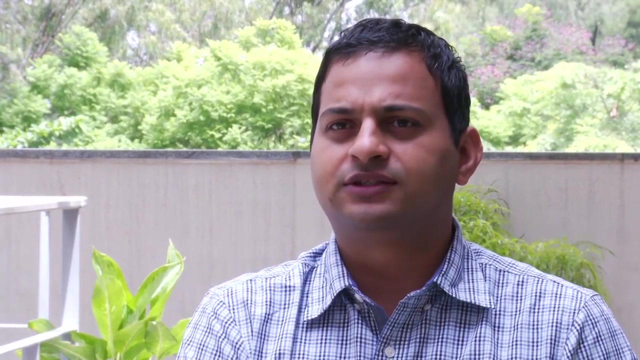 to come to the program, Their backgrounds this year have been quite varied. about 20 percent of them are studying biology and the rest is a fair mix of physics and math, And we also have a couple of students studying computer science. So this school was extremely helpful for me. 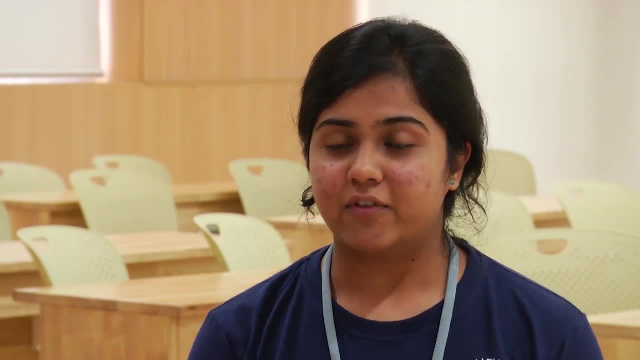 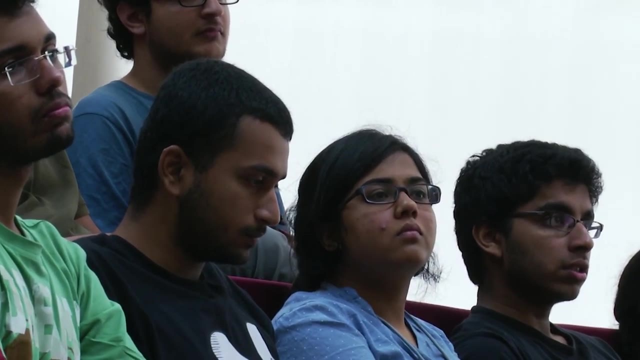 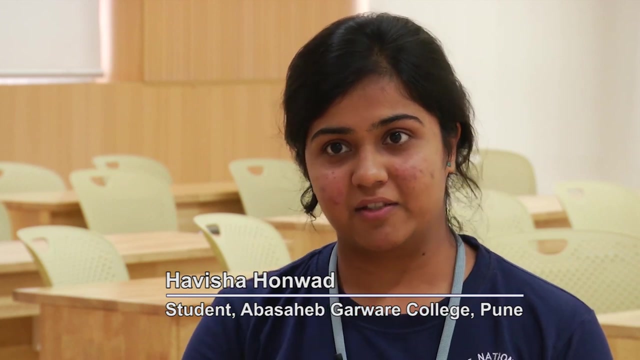 because I have actually now got to know of different areas and basically different streams which are coinciding with biology, to come out with amazing research that is going on everywhere which is actually helping biology come out as a different field. So I'm really glad to be here. 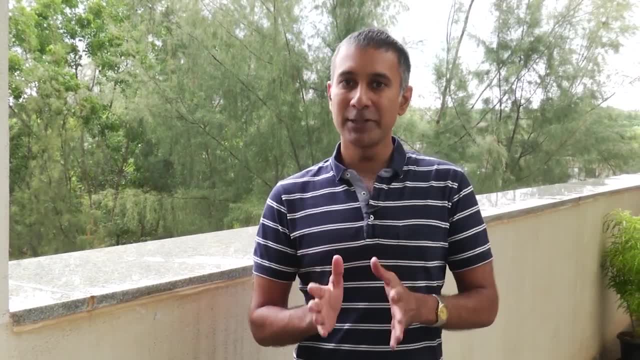 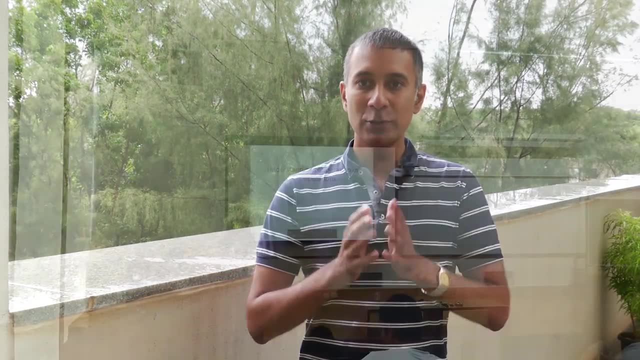 So the Monsoon School consists of really three different portions. One are pedagogical lectures, that is, we give lectures on advanced topics in mathematics, physics, biophysics and so on. Then there's also the so-called research talks, where we invite colleagues from NCVS and other 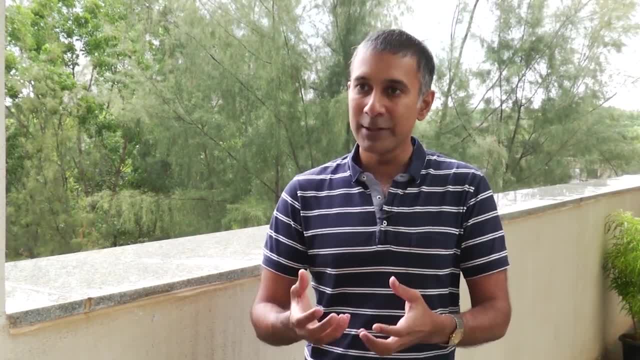 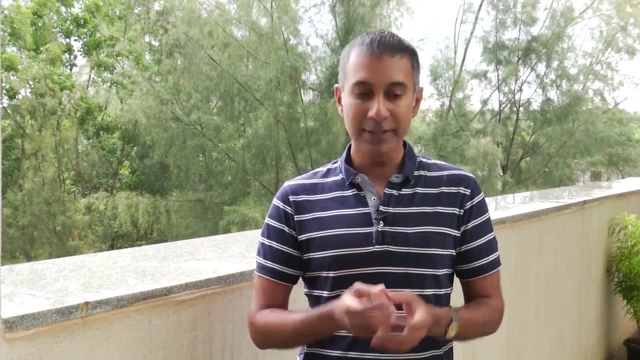 institutes around Bangalore to talk about their own research, real biological questions, the experiments they are doing, And these are at a very high level. Finally, what we have are hands-on sessions, which we call tutorials. Now, these are not experimental tutorials. 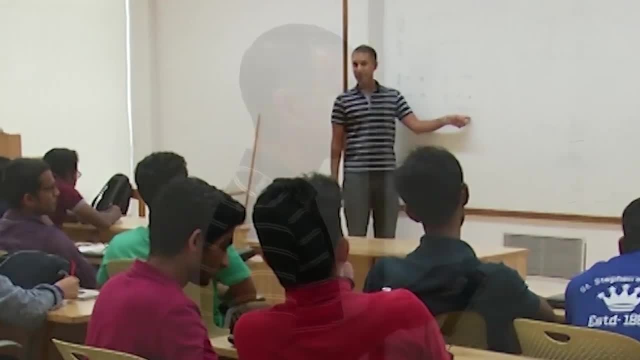 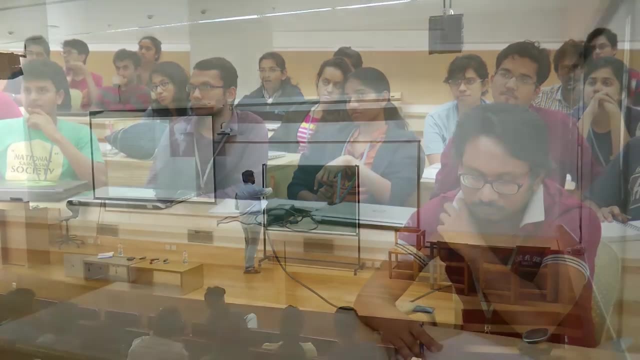 because those are much more difficult to put together. These tutorials: we get the students to actually use the mathematical tools we've trained them on and apply them to questions that they've come up with during the course of the Monsoon School. The idea behind this: 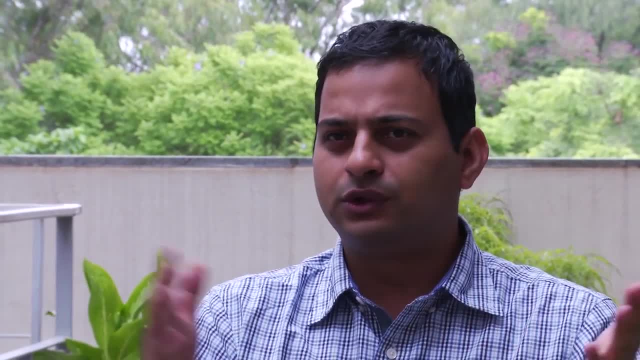 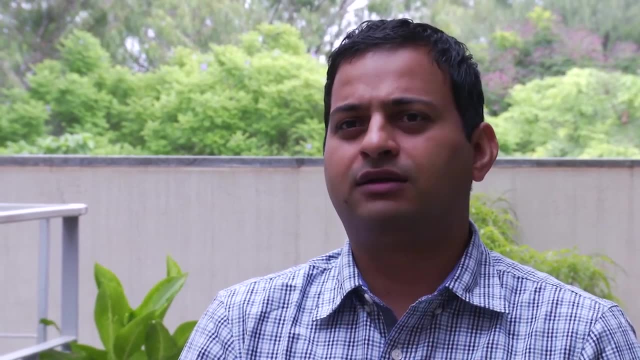 school is really to give the students a window to look at biology in a slightly more interesting way from the perspectives of their training in physics and math and computer science. The Monsoon School is a really great way for the undergraduate students to get a feel for the kind. 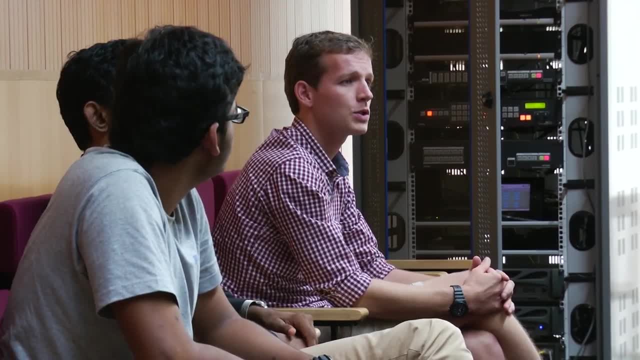 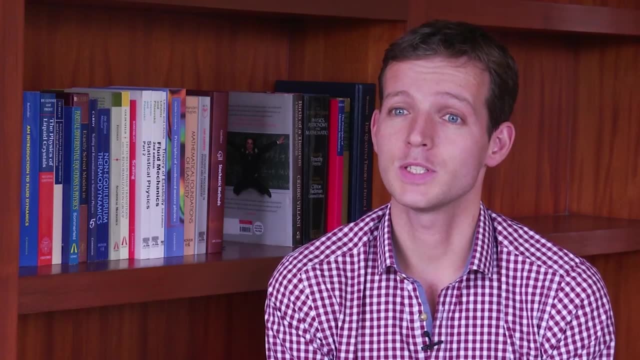 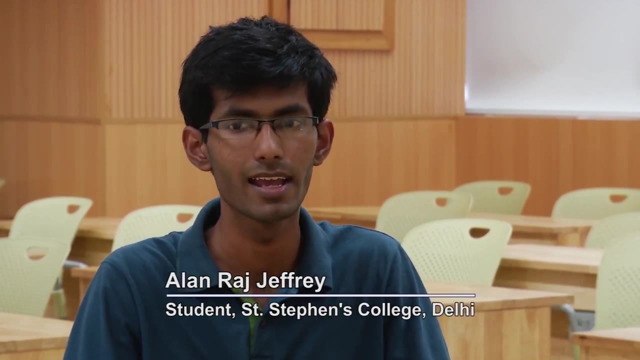 of research that we do here at NCVS, and especially for those who are working in mathematics, physics or computer science, to really understand what their role for these kind of researches are in modern interdisciplinary biology. I've never been exposed to all these other fields of biophysics. 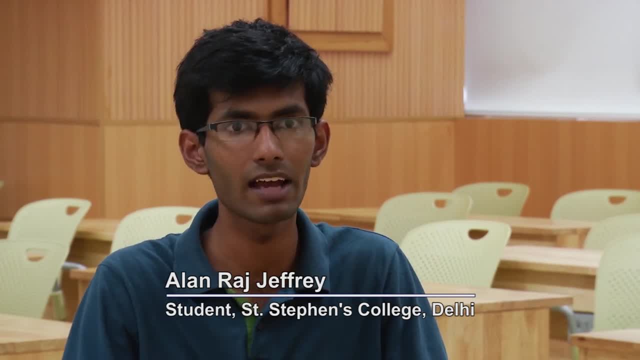 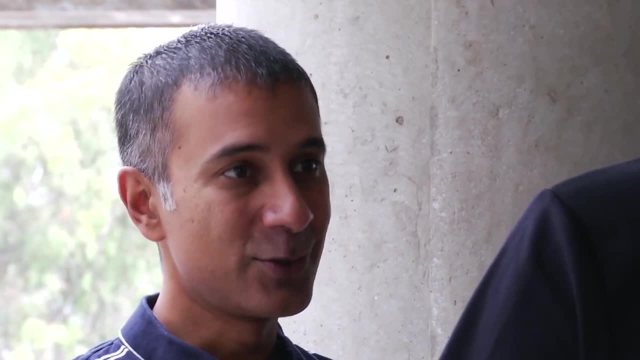 and now I have so many people who I can contact if I have ideas. So in that way, this Monsoon School has been very good for me And apart from that, the conversations that we had, each conversation that we had, I get like 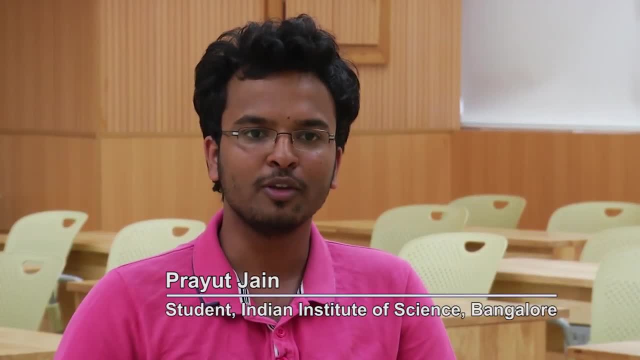 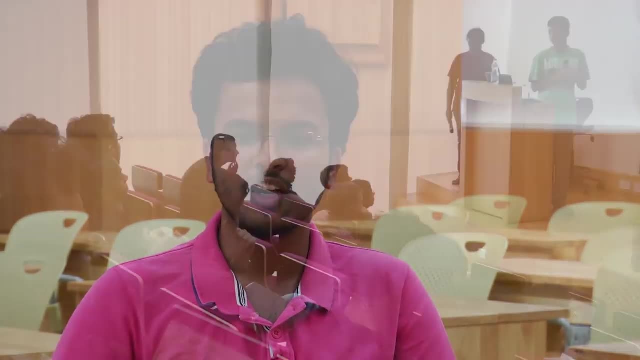 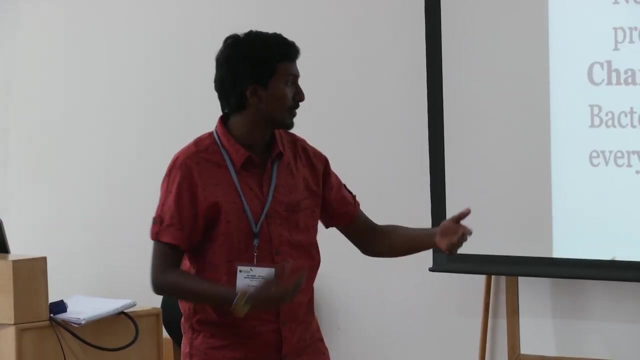 five different ideas from this. The profs over here, like we used to sit for lunch together and we used to discuss stuff like open-end problems- were given to us and interactive sessions were there. So profs are really nice and it was an awesome experience. So I think one of the most 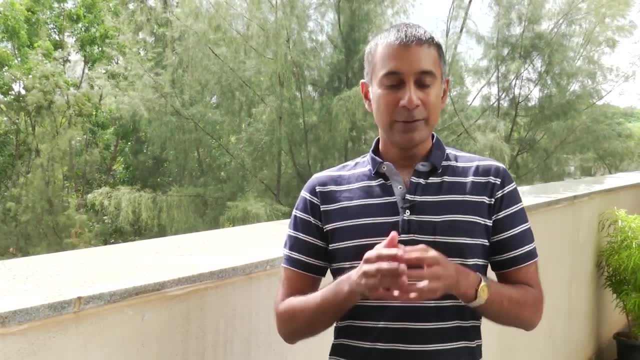 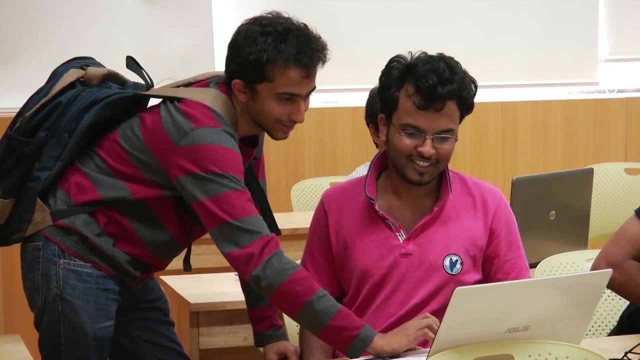 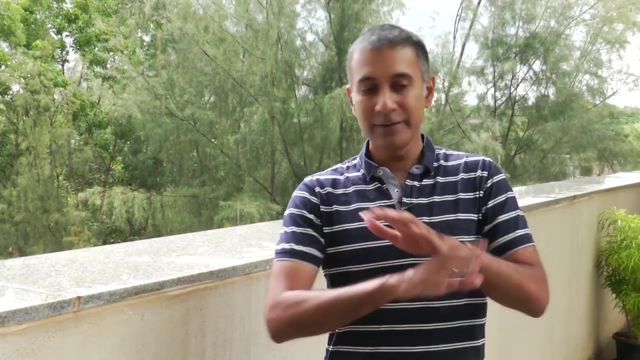 important ingredients of the Monsoon School is the idea of student projects. What we do is on the campus, we ask students to break up into groups of about four or five and we try and mix people between different institutions And we ask them to brainstorm and think about defining an open 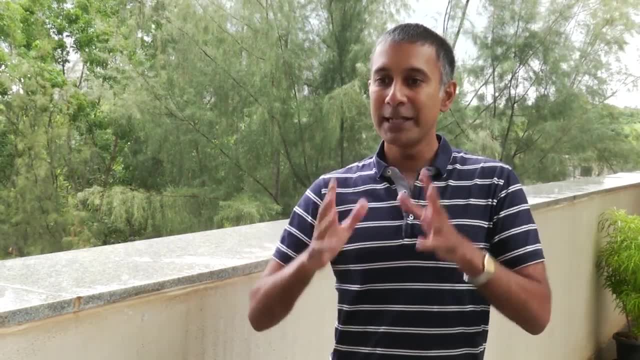 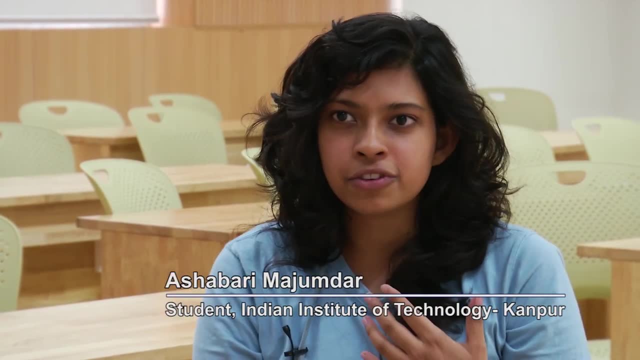 quest. It doesn't matter if somebody else has solved it before. the idea is just for them to be creative and come up with something. Best thing about this school is, like I got to know that it doesn't matter like from which stream I am from, I can apply my skill to. 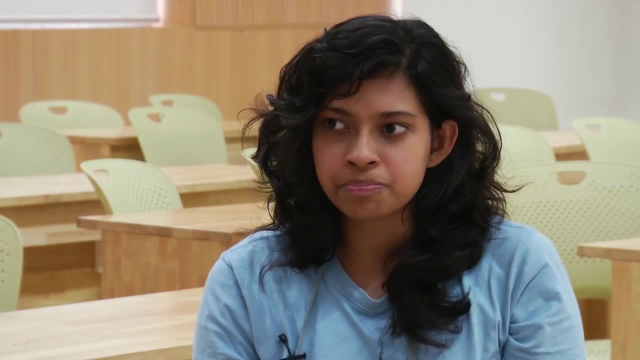 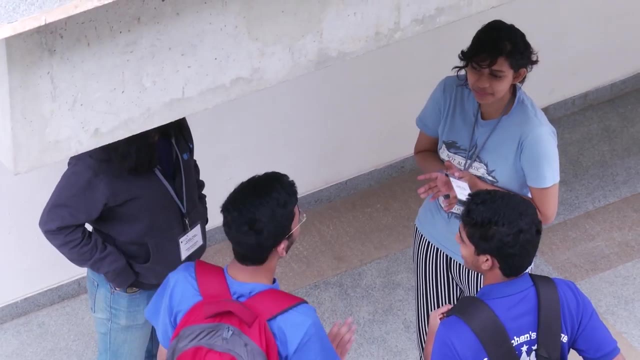 any of these interesting biology problems. Lots of problems, active problems are in the school so I can like join and explore this field. That's the best thing I which I got here And the other things are like I got to know. 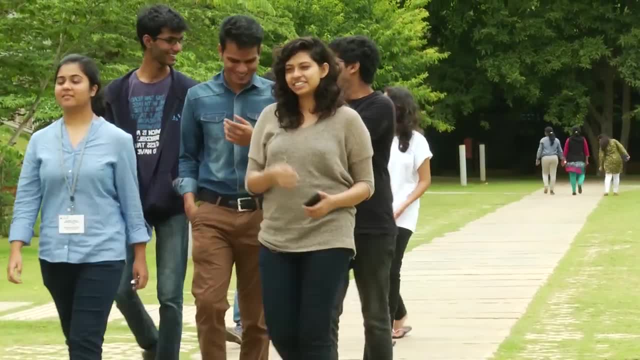 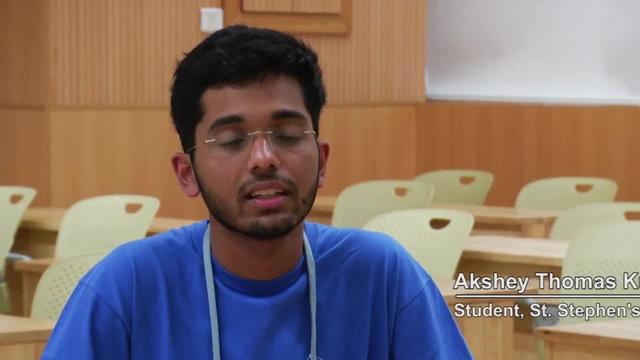 like lots of people from different background, different colleges from all over India, So I had a really good experience here. So coming to this NCBS like it opened a whole range of new questions to me, So that was very interesting. I. 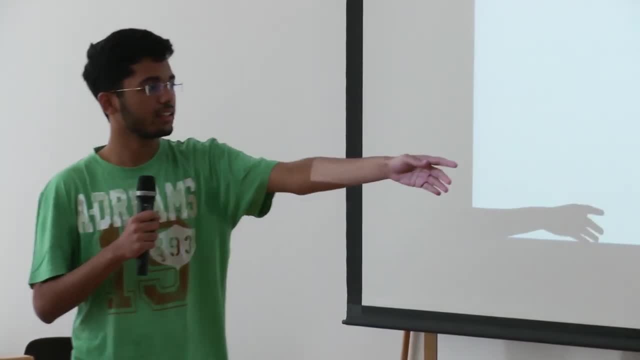 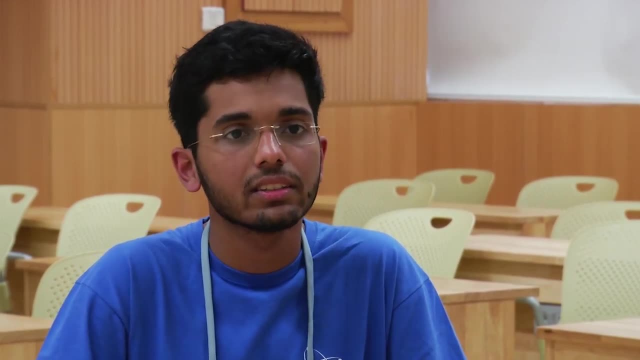 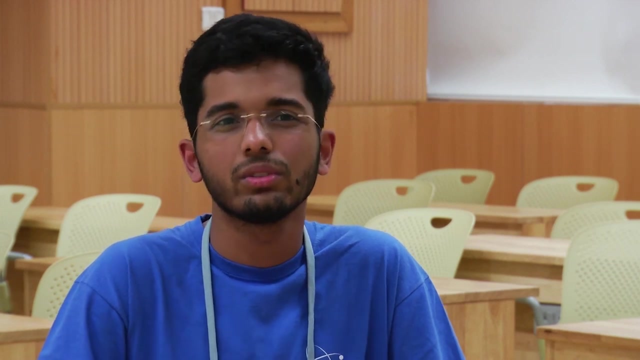 also enjoyed the fresh approach that these people had to biology, even though many of them came from maths and computer science and physics. I found that very inspirational in a way, because we weren't tackled to manage normal problems. I mean we usually had to say, okay, a biologist tackles.